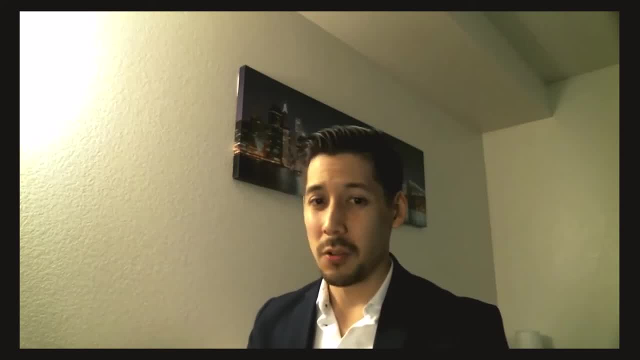 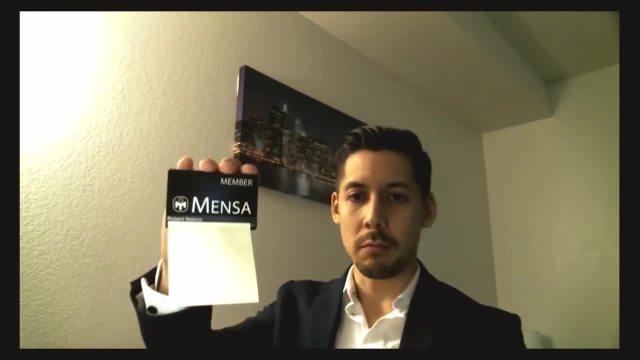 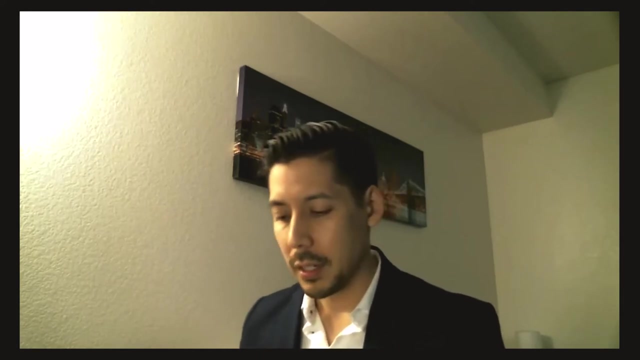 California. I took the test. There were about maybe like eight other people in the room also taking the test And, lo and behold, I passed. So here's my Mensa ID card. You can see my name's on it, But I covered the ID numbers so that you can't make a fake copy and pretend to be me. 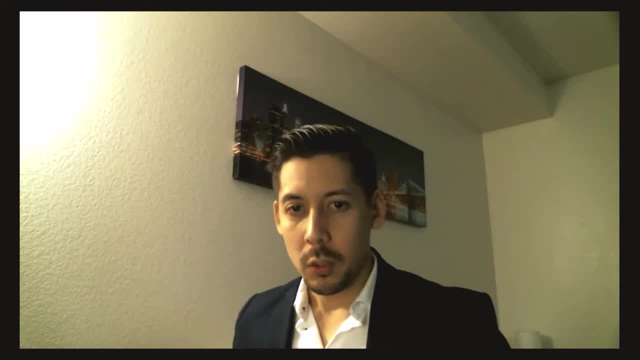 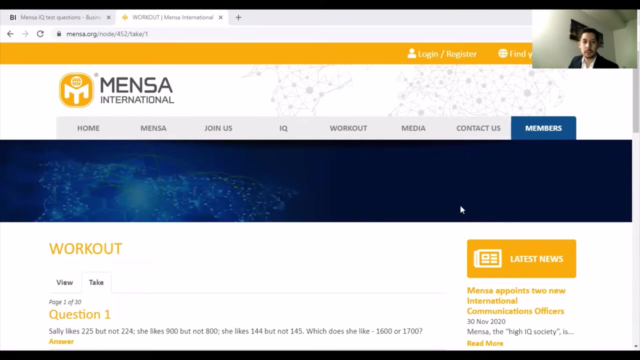 That being said, let's jump into. what did some of these questions look like? How did I prepare for it? And then I have a word to say on how emotions are actually more important than intelligence. But let's get into it. So what you got to do is go to the Mensa website. 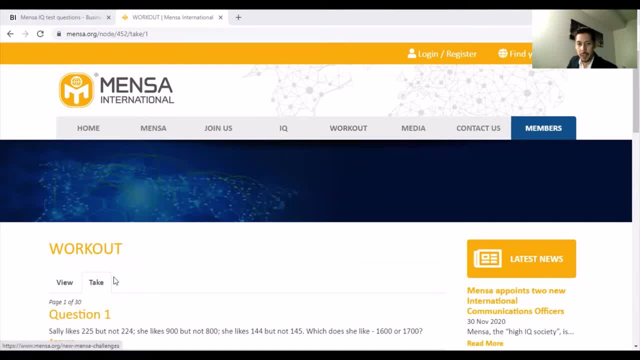 Mensaorg. Then you click on Workout New Mensa Challenges And you click on the 30-question workout. They used to have like a sample test, I think, And I don't see that right now, But this workout has some of the same questions from that sample test, So let's go through some of them. 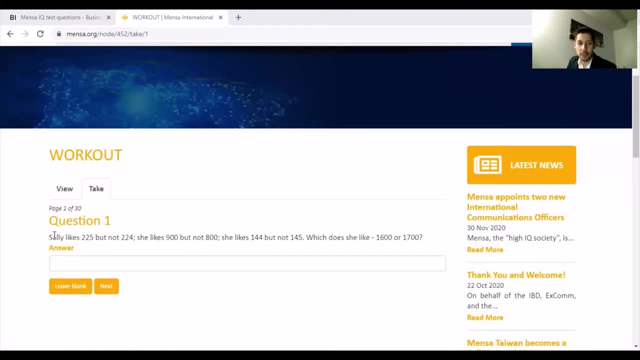 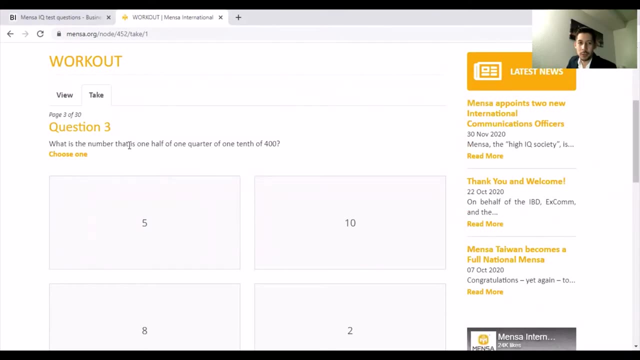 not all of them, because some of them are boring, to be honest. Like that one's boring. A lot of the math ones are boring Because you just do, you just write algebra equations to solve it, Like this one. What is the? 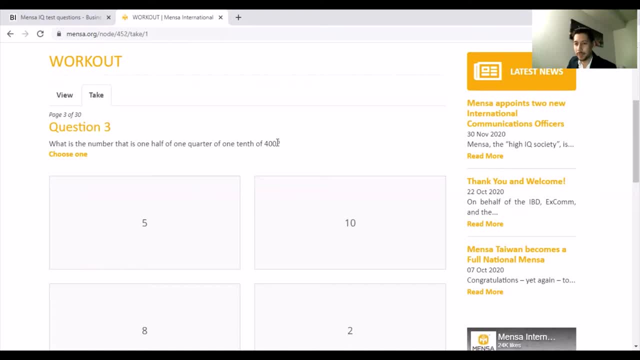 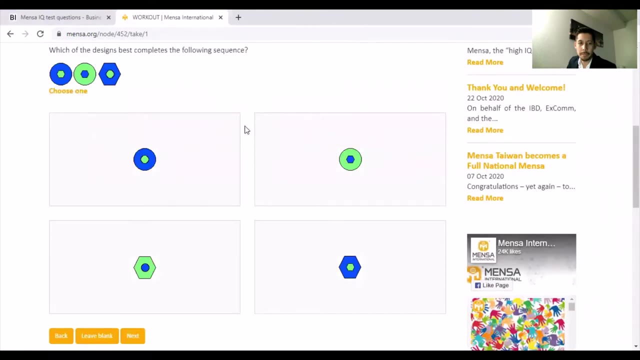 number that is one, half of one quarter of one, tenth of 400?? Well, 400, a tenth of that is 40.. A quarter of 40 is 10.. Half of 10 is 5.. So there's the answer. Boring question. Okay, here's, here's. 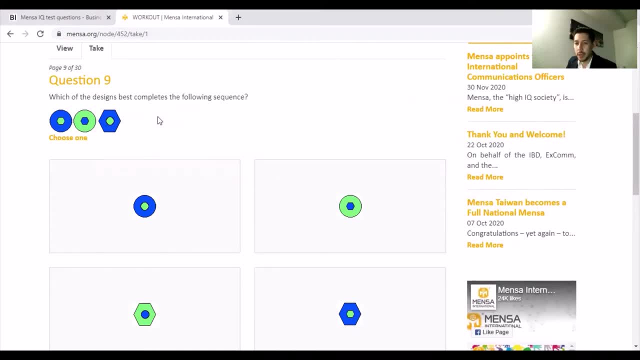 one that I remember seeing, A type of question that I remember seeing on the exam when I took it: Which of the following designs best completes the sequence? So you got to figure this out. Well, it's green in the middle, then it's green on the outside, then it's green in the middle, So it should be green on the outside. 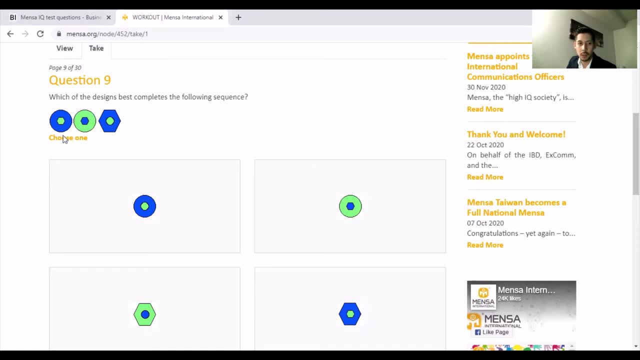 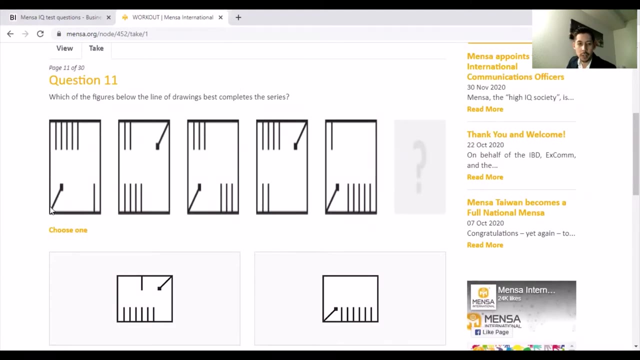 But there's two of them. So how do you pick which one? Well, this is a hexagon, hexagon, circle, circle. So that one. Next, Another good figure, one. Okay, So this little weird thing goes from here to up there, then it goes. 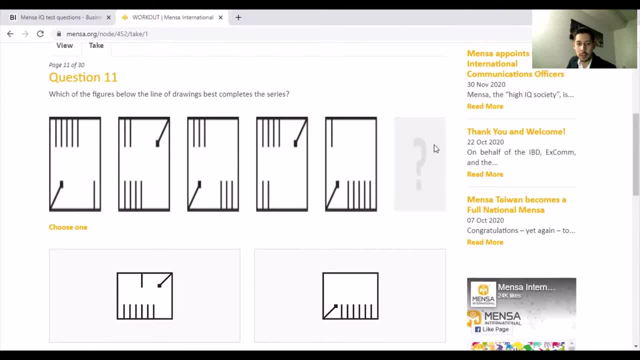 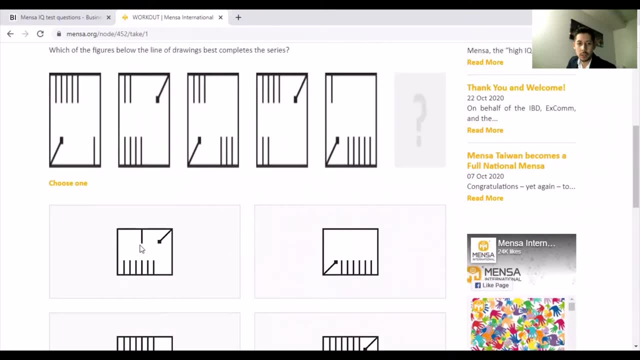 down, then it goes up, then it goes down. So it should be up again, But there's two answers that have it up there. So then you have to look at what's the meaning of these things, Right? Well, you have 1,, 2,, 3,, 4,, 5, then it goes to 3, and then it goes down to 1.. It only applies to the. 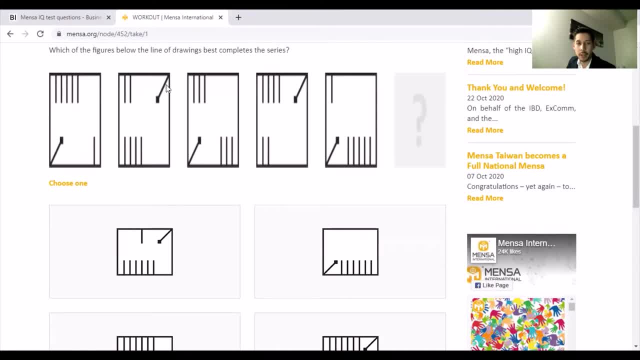 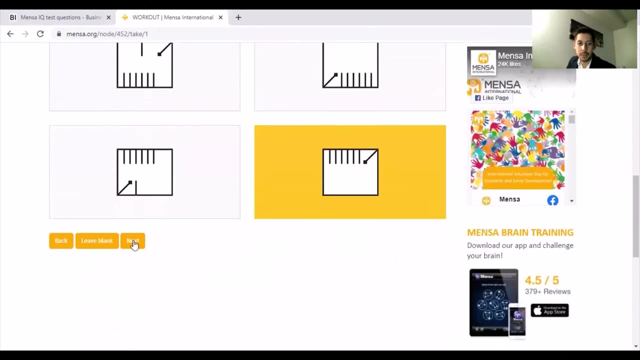 ones where the this little lever thing is down. If it's up like that, it goes 2, 4.. So I would expect either 6 or 8. Definitely not 1.. This one has 1,, 2,, 3,, 4,, 5, 6. So I'll go with that one. Fill in the missing number. First I thought like 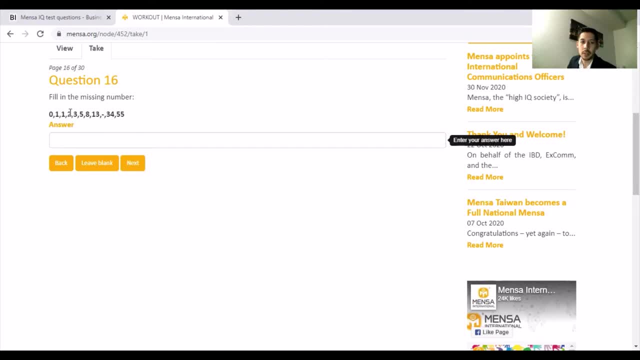 oh, it's, the each number is the sum of all the numbers before it, because 0 plus 1 plus 1 is 2.. And then, but I, when I did 3,, 3 is 2 plus 1 plus 1.. No, that doesn't work. 2 plus 1 plus 1 is 4.. 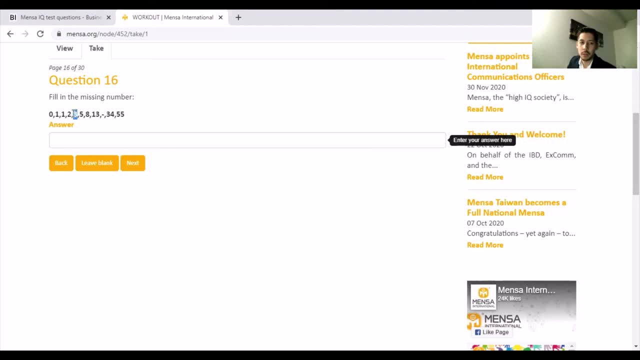 So then I was like: so what is it then? So maybe it's just that the 1 plus the 2 is the 3.. So then 5 is 5, I realized is 2 plus 3.. 8 is 3 plus 5.. 13 is 5, 5 plus 8.. So it's just the sum. 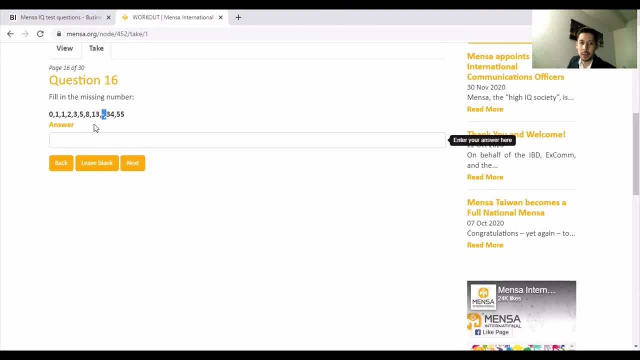 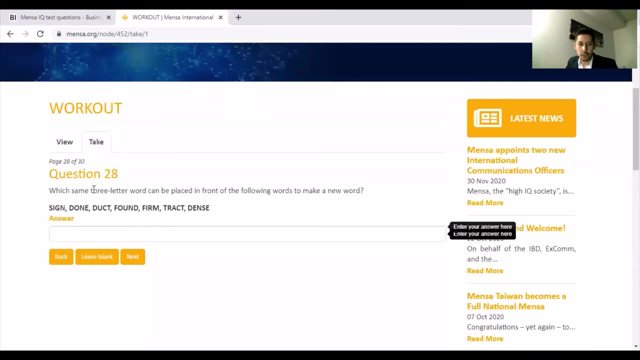 of the last two numbers, So 8 and 13.. You add those together and it's 21.. Which same three-letter word can be placed in front of the following words to make a new word? So, because this was three, I was thinking re-sign. but no, that's two letters, not three. 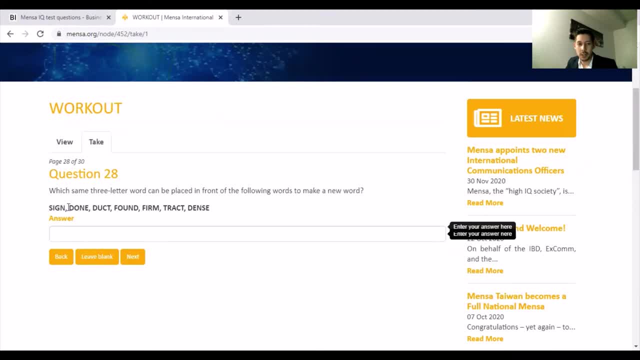 So undone is a word, but that's two letters. Duct makes me think aqueduct, but that's four letters. Found is a very general firm. Then I thought: oh, confirm, C-O-N. So does that work? Contract, condense, confound. conduct, condone, consign. 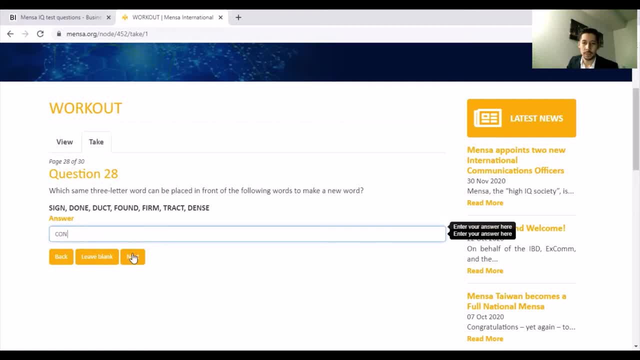 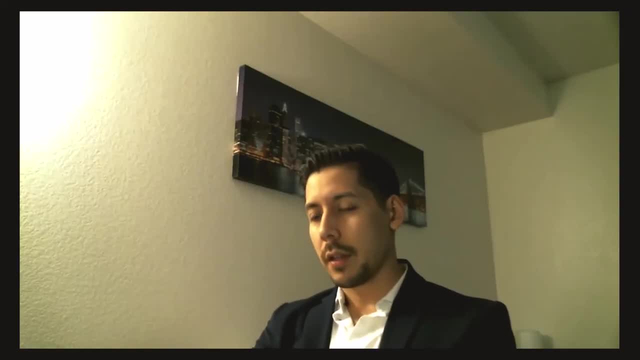 Yes, that works. So C-O-N is the answer. When I got into Mensa I started going to some of the other places, some of their gatherings. They had little get-togethers at people's houses. I went to these houses of random people I didn't even know. 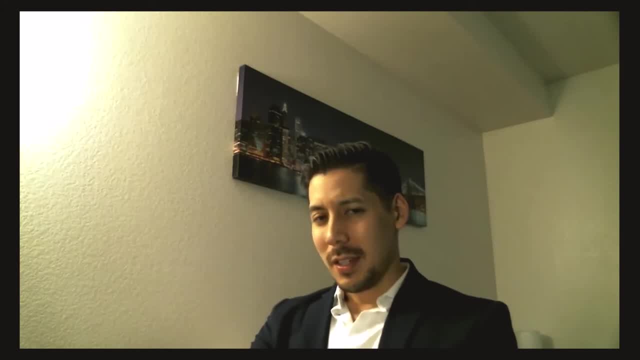 And what else. Oh, I met up with them at Starbucks And what I can say is that intelligence, yeah, it's valuable, but it's not everything. And one thing that I really admire about people is emotional toughness, emotional fortitude. 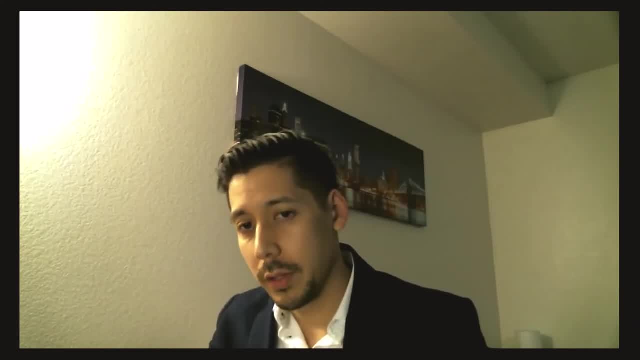 So now I'm going to play an excerpt from an audio book. This is a business audio book that I've been listening to, written by a very, very successful person, And what he's saying here is that he knows a lot of intelligent people. 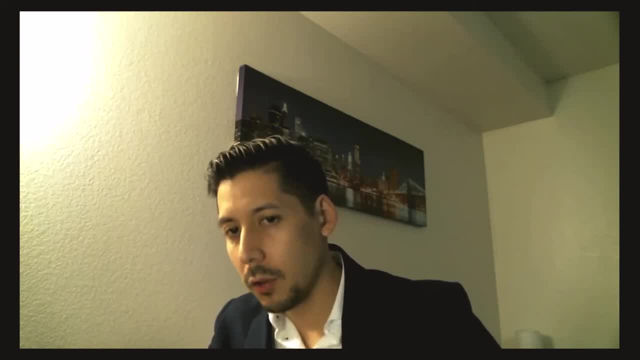 but because they don't have the emotional toughness, the ability to handle pressure, they don't succeed as much as he does. It's very insightful and so take a listen. I've had some very smart friends who I have kept in touch with. 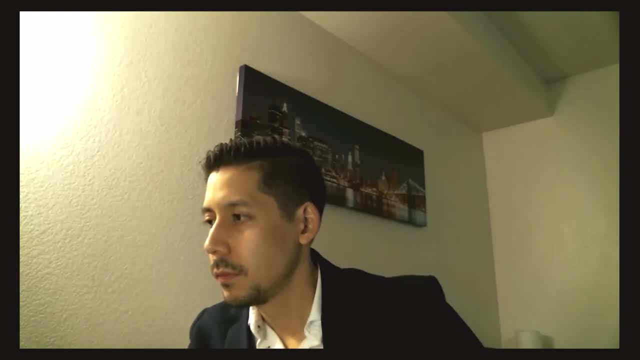 one person in particular was a total genius and he never made it. He has a nice job working for an accounting firm, but he went out recently to buy a house and he was a basket case. He called me and asked: do you think I'm making a mistake? 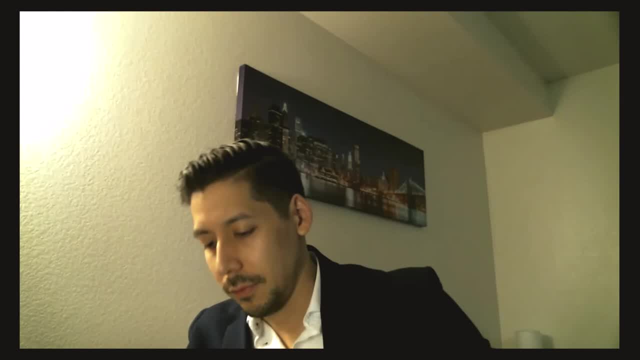 I don't know what I'm doing. I'm so nervous. I'm buying a house. I mean, what do I do? Do I borrow? He was devastated over the fact that he was buying a house. After he bought the house, this brilliant guy called me and said: 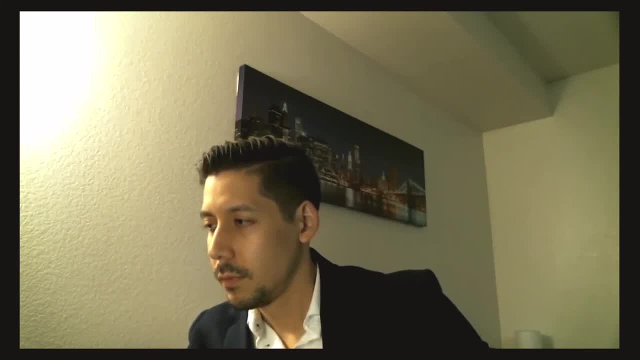 I bought a house. Do you think I did the right thing? I have a mortgage. Oh my God, will it be all right? Here's a guy with a lot of money, He has a 180 IQ and he cannot sleep. 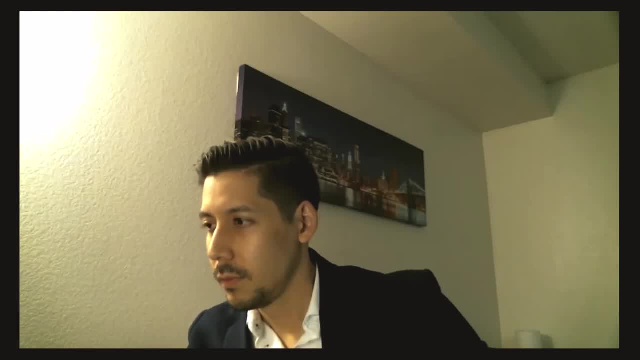 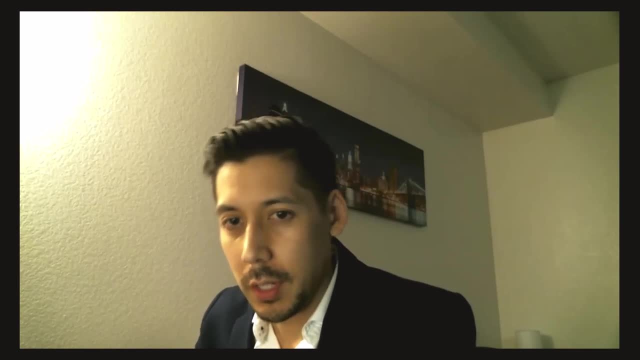 and he cannot have sex with his wife because he's so stressed. All right, so that's an example of how emotions need to be handled, and that's the whole point of this channel existence. first, is I, as a human being, want to use my intelligence to take control of my emotions. 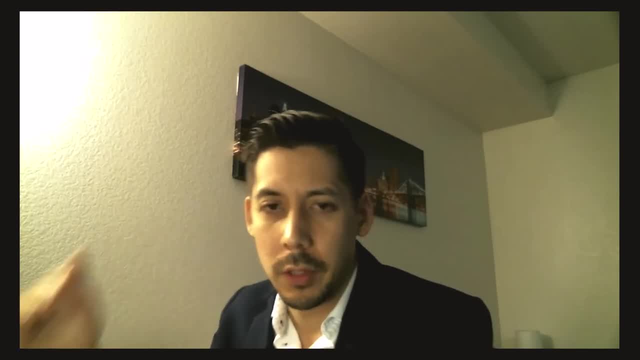 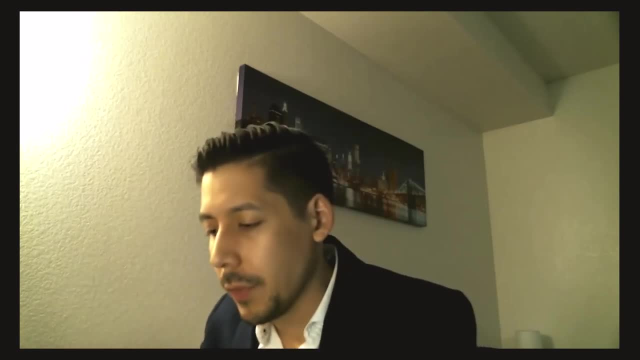 and then taking control of my emotions controls my physiology, Outer brain, limbic system, outer brain, emotional brain and reptile brain, And that's my philosophy. I mean, I want to look up to humans and I want us to use our intelligence.